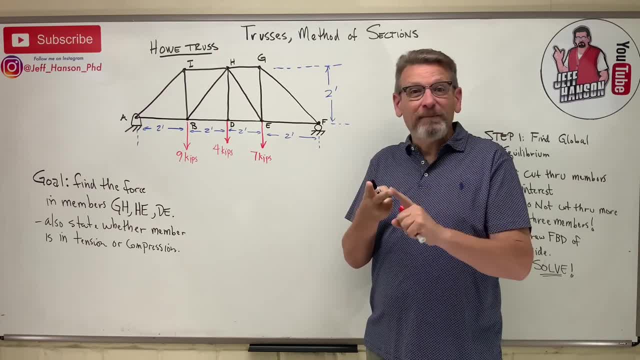 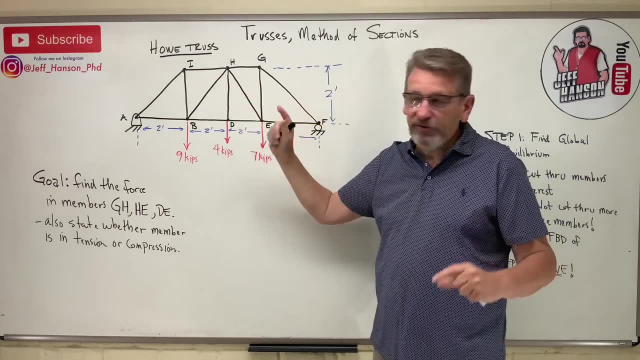 about the method of joints and today we're talking about the method of sections. okay, The method of sections. I have a truss for you here. This is called a Howe truss. That's just the guy that designed this particular truss, And they want us to find the force in members. 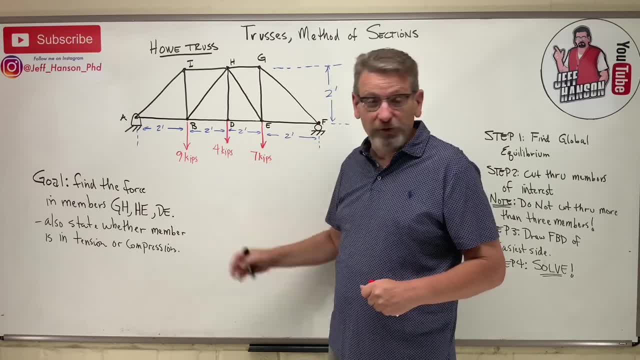 G-H-H-E-L-S, G-H-H-E-L-S, G-H-H-E-L-S, G-H-H-E-L-S- In D-E, and also state whether those members are in tension or in compression. As you know, when we do truss problems- that's a new thing for us- We have to tell whether it's in tension. 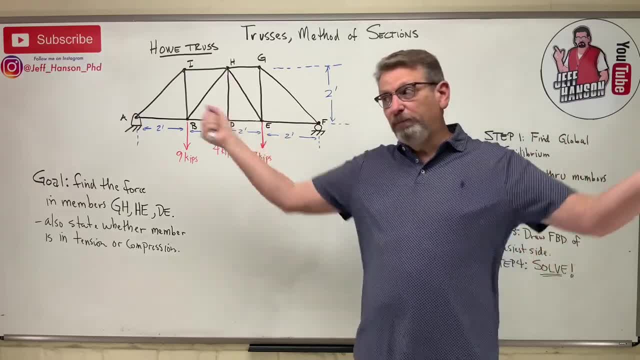 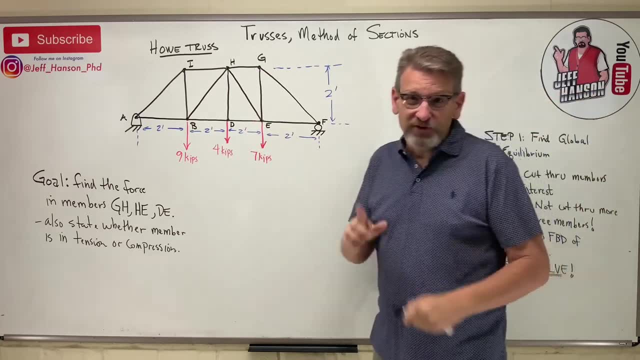 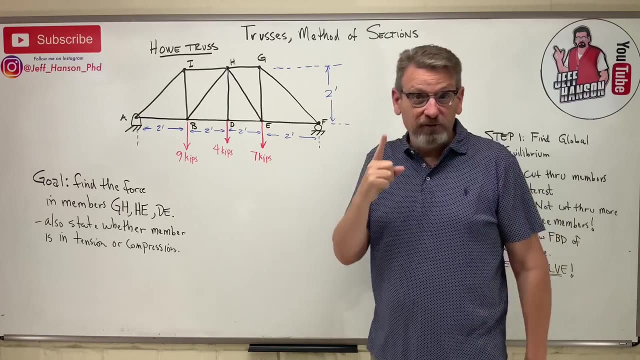 or compression. And remember, tension members are always pulling on the joint and compression members are always pushing on the joint. okay, So first question: How do I know to use the method of sections or the method of joints? How do I know? The answer is simple: If they ask you for. 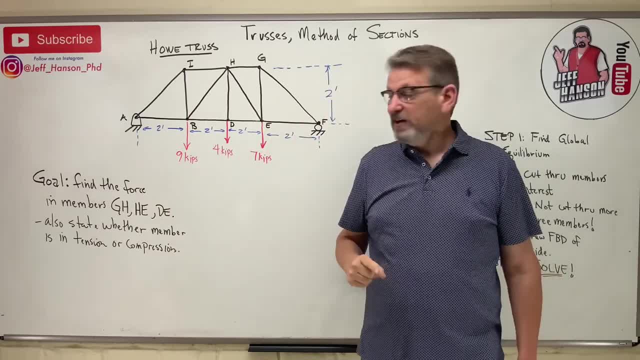 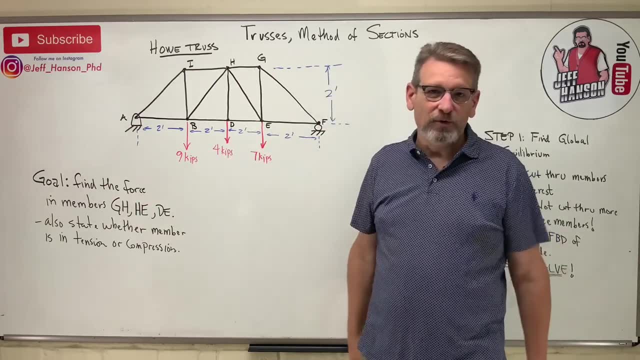 members, then you need to be thinking to yourself. method of sections: If they ask me find every member in the truss, then I might as well use the method of joints. That's the easiest thing to do, okay? So how do you use the method of sections When you see particular ones? okay, 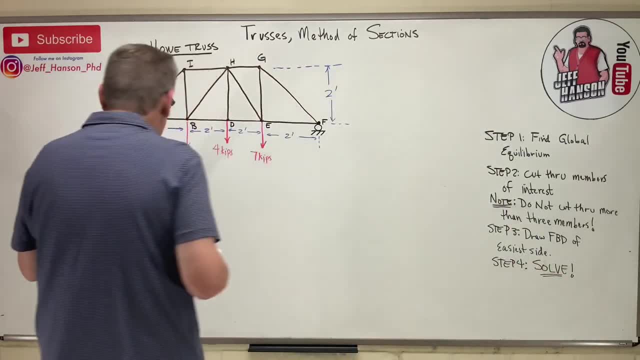 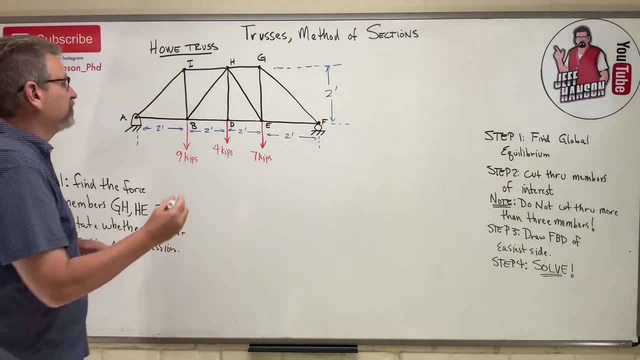 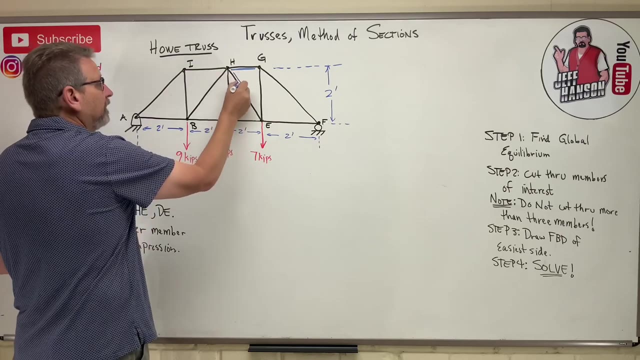 And what I like to do here is highlight the ones that they're asking me about. So they're asking me about G-H-H-E and D-E. So here's G-H up here. I'm just going to kind of make them blue, okay. So that one. H-E is this guy, okay, And D-E, which is this one here. 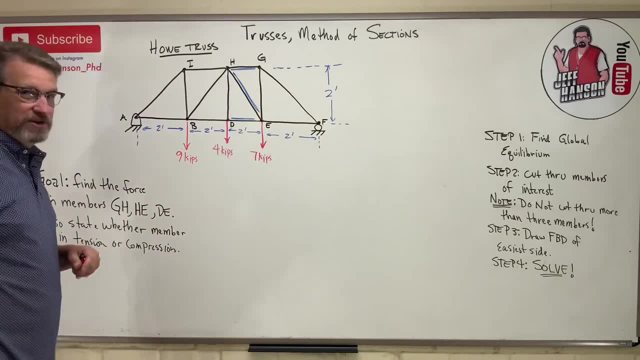 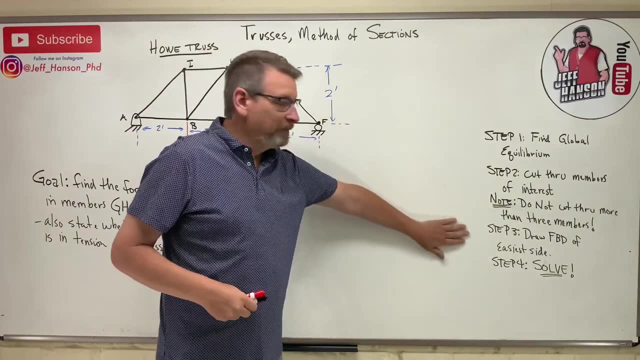 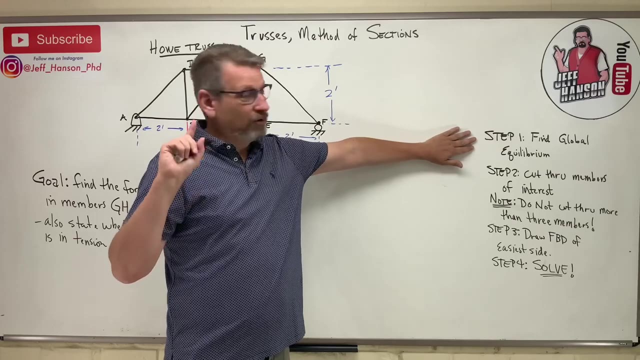 okay, Just to kind of remind myself which members they're talking about. okay, So I have written you a recipe over here. We like recipes, don't we? If you follow this recipe, you can do method of sections. Piece of cake right. Step one: find global equilibrium. okay, Now, global equilibrium. 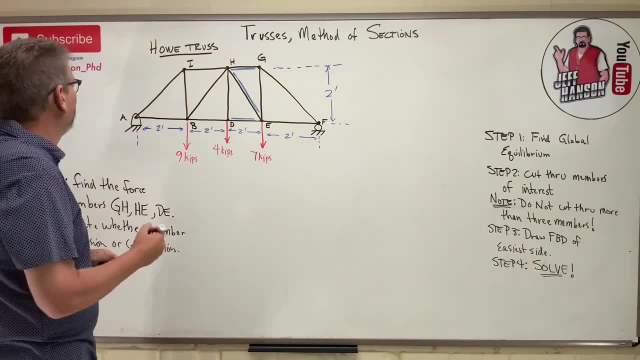 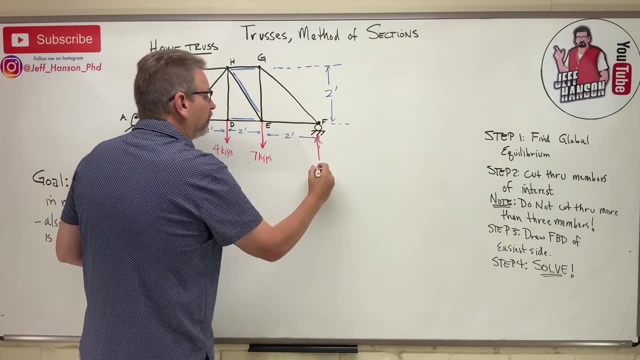 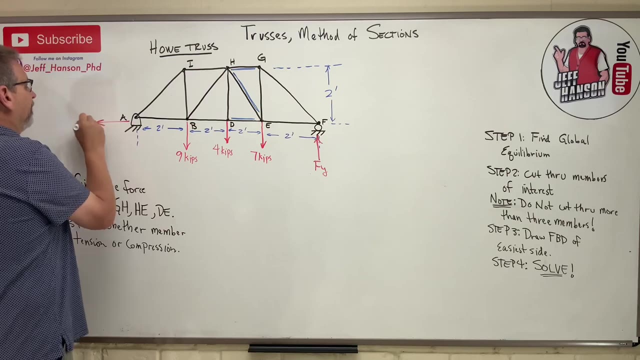 forces. okay, So where this thing is hooked to the globe, where is it hooked to the globe? At point A and point F. okay, Over here at F is a roller, So guess what, There's a normal force over there. We'll just call him F-Y. And then over here is a pin connection. okay, It's got an A-X. 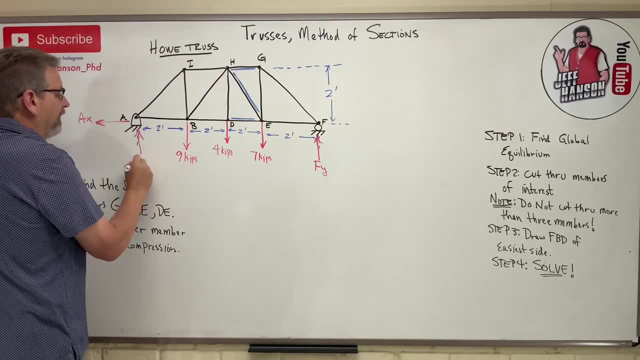 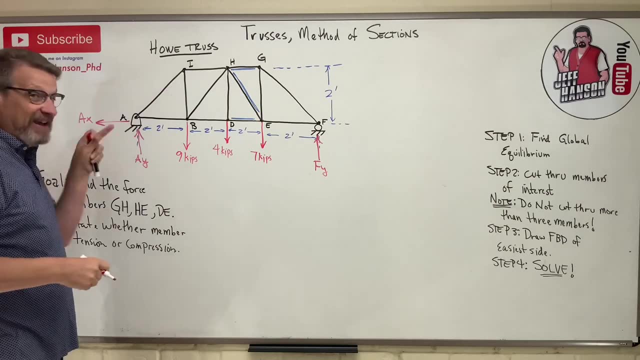 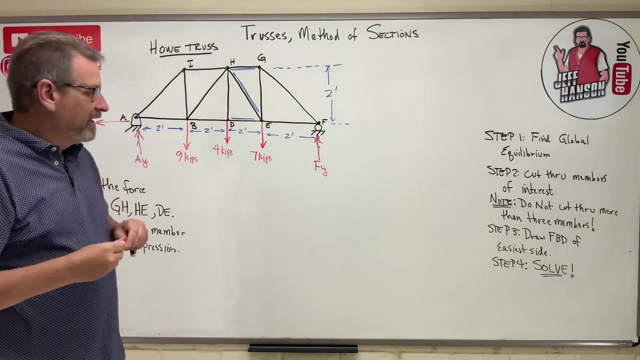 and an A-Y Now, right away. I don't see any forces in the X direction, And so this is like a good friend over here. He's there when we need him. We just don't need him right now. okay, So he's zero, okay, So how can I find A-Y and F-Y? 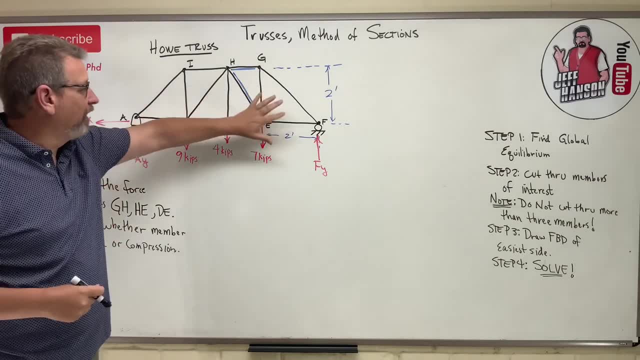 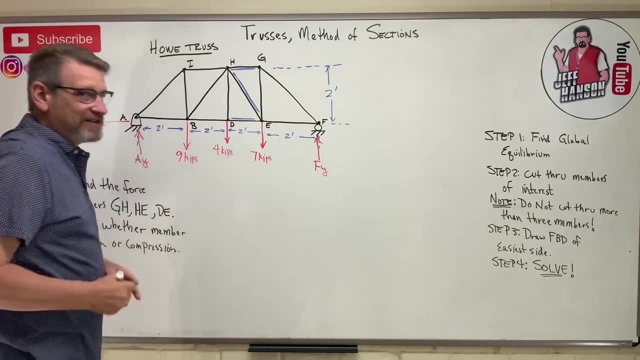 okay. Now, since this is a symmetric truss, if the load was symmetric I could have just divided in two and said: okay, you got half and you got half, But the load is not symmetric, And so we're going to have to write a moment equation. So I'm going to go up here and do global, okay. 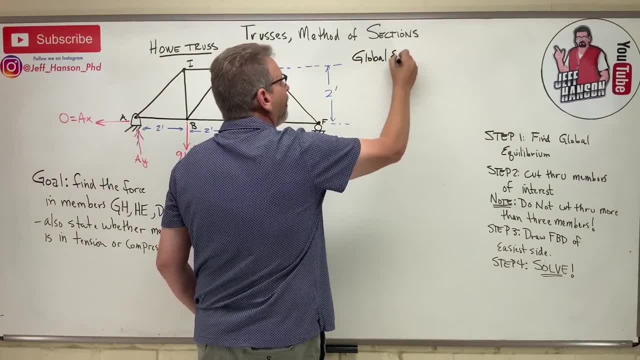 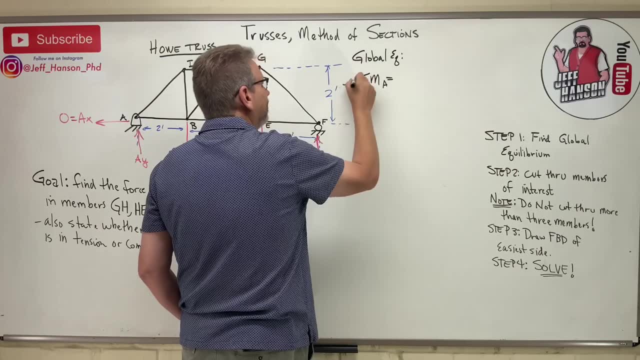 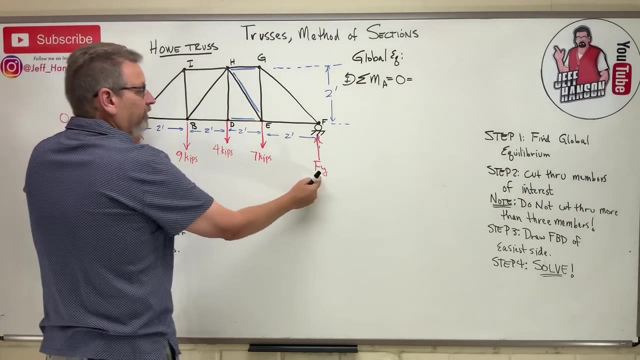 So here comes global. okay, And what I'm going to do, I'm just going to take the moment at point A, okay, This being positive, okay, So I'm going to take the moment here, okay, And I get, I'm going to go over here first, F-Y. 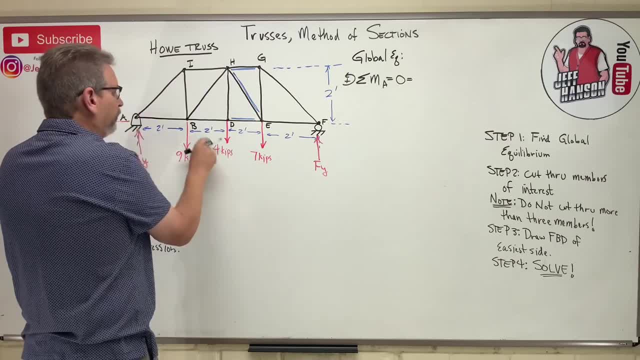 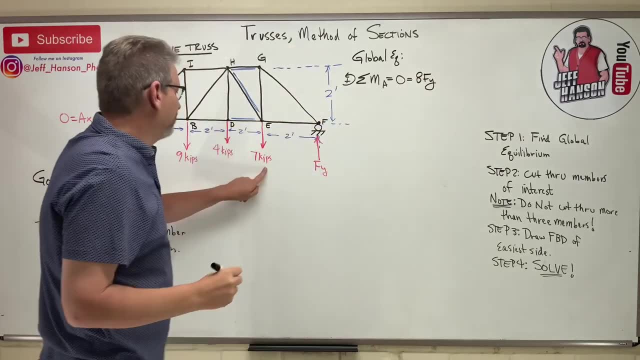 whoop rotating me positive, So F-Y times 2,, 4,, 6,, 8.. So 8 F-Y. And then the 7 is rotating me negative right Times 2,, 4,, 6.. So 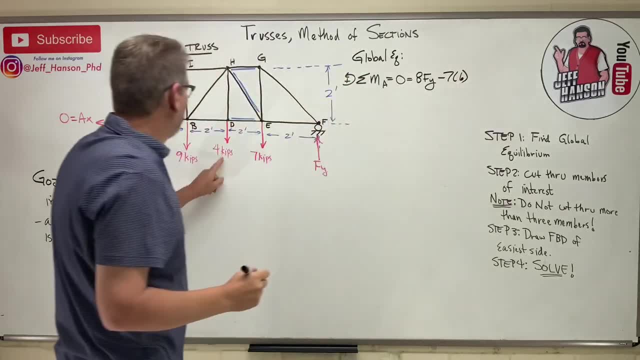 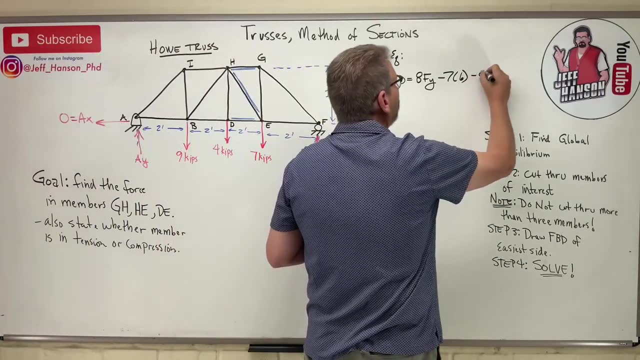 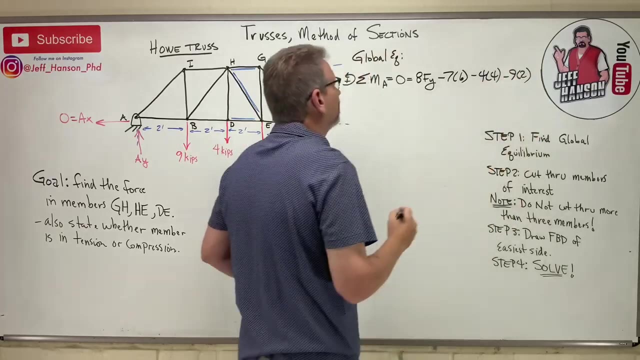 minus 7 times 6.. And then the 4 rotates me negative. The 9 does too, doesn't it? So 4 times 4.. So minus 4 times 4, and also minus 9 times 2, okay, So what is that? All right. 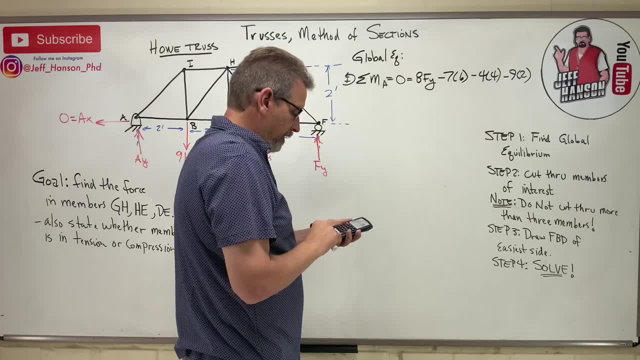 here we go On: clear 42 plus 16 plus 8.. So what is that All right? here we go On clear 42 plus 16 plus 8.. So what is that? All right? here we go On clear 42 plus 16 plus 8.. So 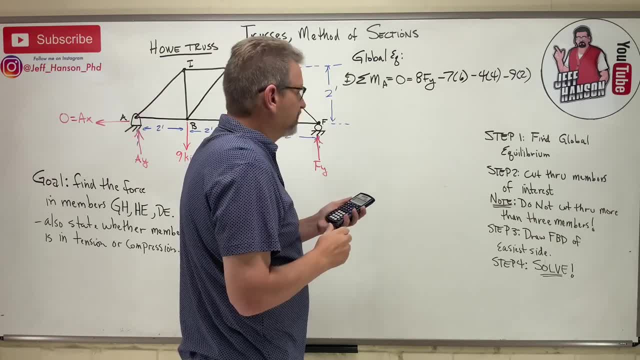 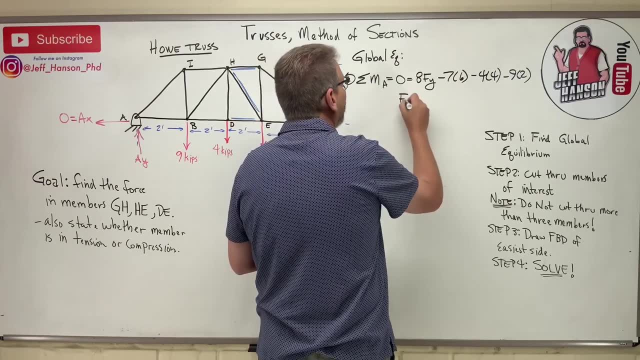 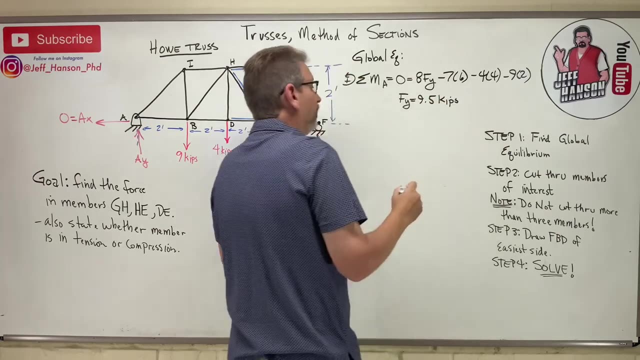 18 equals 76. divided by 8 equals 9.5.. So F-Y equals 9.5.. And that's a kips which we know is a kilopound, a thousand pounds right. And so the total downward stuff is 9. 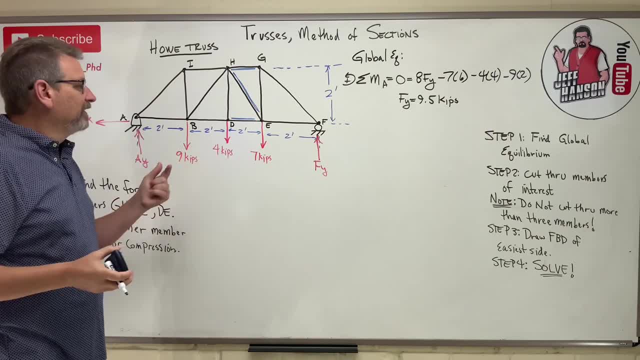 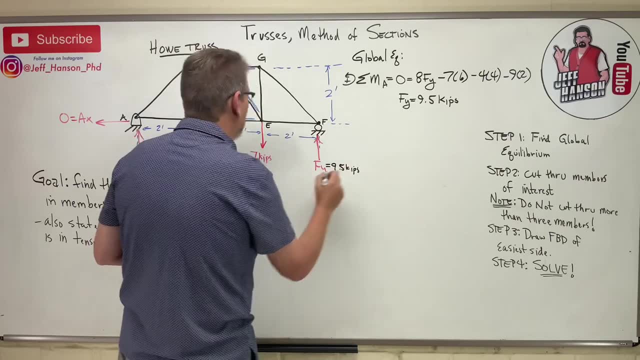 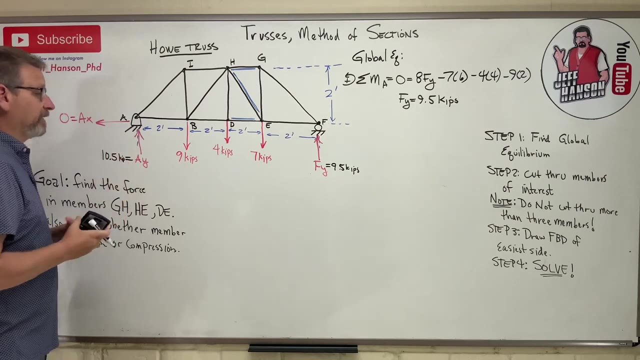 plus 7 is 16 is 20, right. So the total upward stuff has to be 20, right? So if this guy's 9.5, okay, then a Y has to be 10.5, okay, Because 10.5 plus 9.5 is 20 going up. and then I got 20. 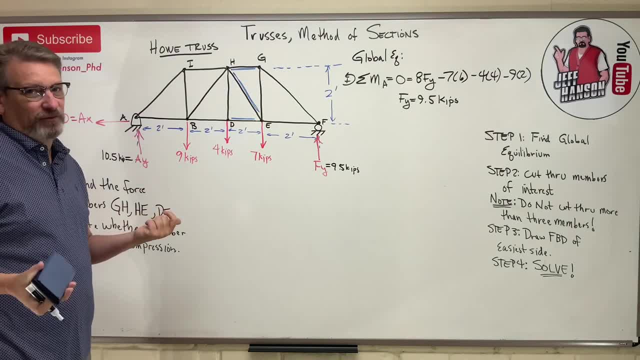 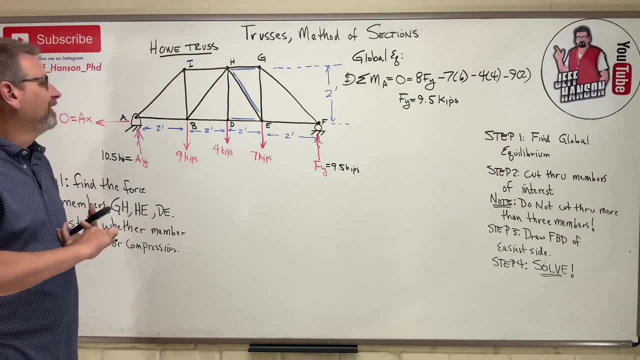 going down, okay, And all that is is the sum of the force and the Y. That's all that is. I just did the sum of the force and the Y in my head because I'm like super smart, okay, Next bit. 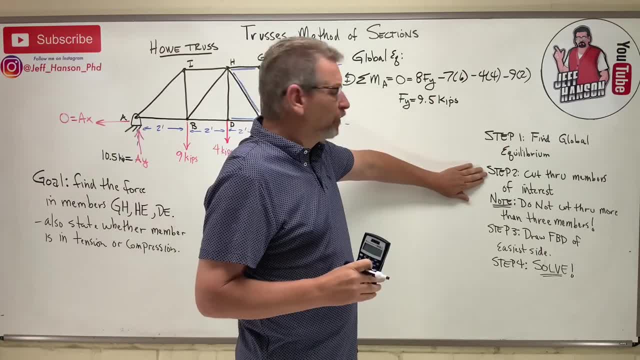 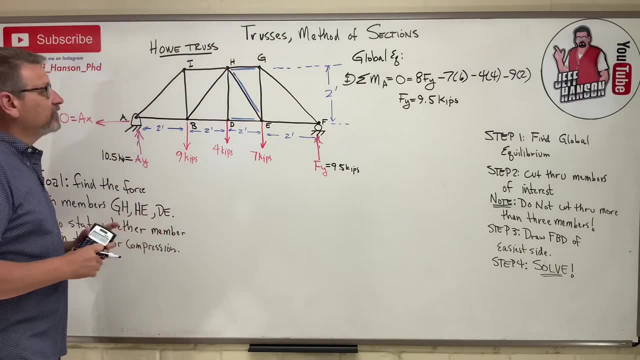 okay, Step two: cut Cut through the members of interest. Now, the members of interest are these ones that they want us to find over here: G-H, H-E and D-E. So I'm going to make a squiggle cut line. I'm 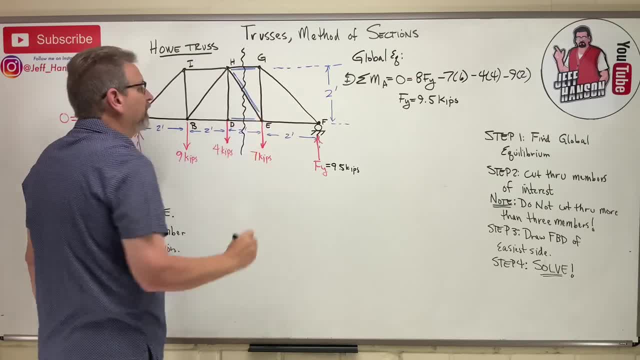 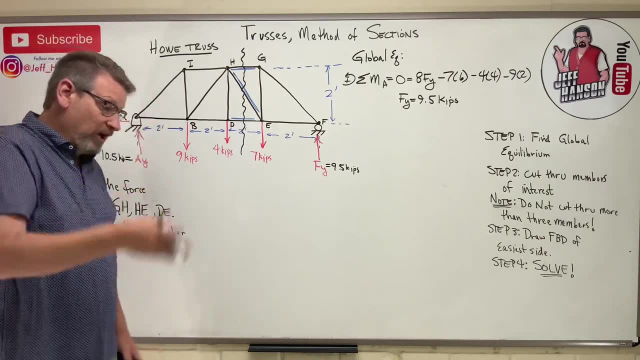 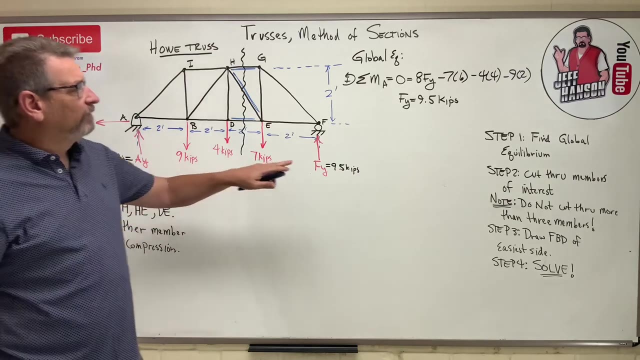 going to cut the truss through there. okay, Now, to section something means to cut it. okay, If I go out and section a beam, then I cut through the beam and I look at the cross section of it where I cut it in half. All right. So it says: next cut through the members of interest: No. 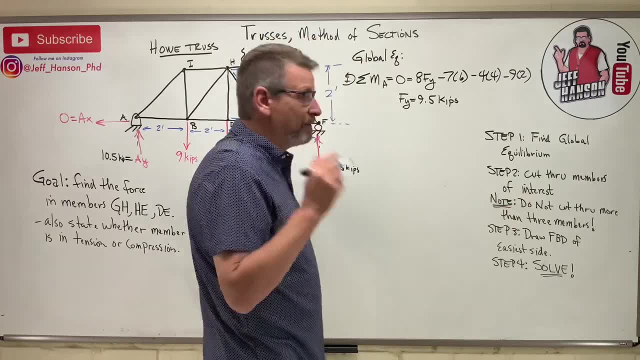 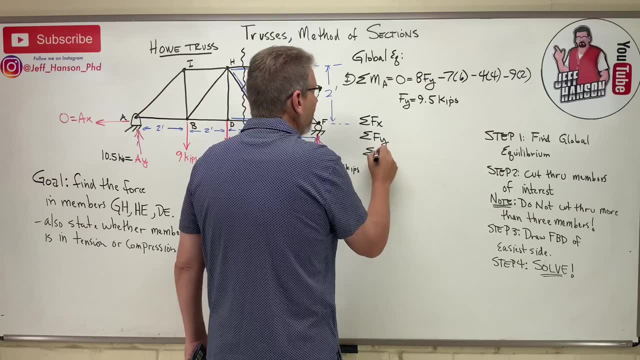 do not cut through more than three members, because in the method of section we have this: the sum of the forces in the X, the sum of the forces in the Y, and we now have the moment, is back. okay, So that's about some point. I don't care which point you pick, I shouldn't put A I. 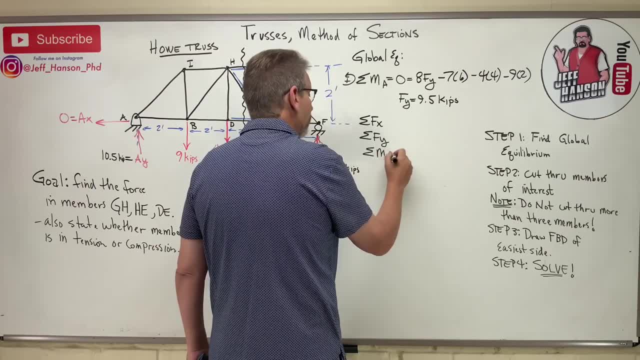 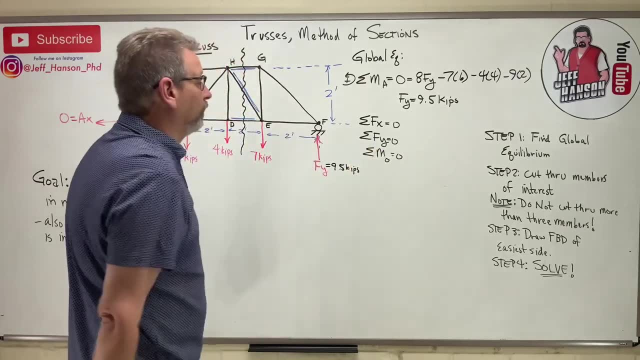 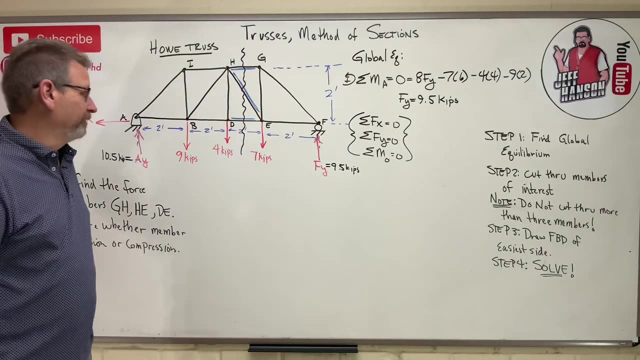 should just put O for just whatever point you want, right? So those are the three equations that we have available to us. So if you cut through more than three, you're not going to have enough equations to solve for it. So in this case, I cut through one. 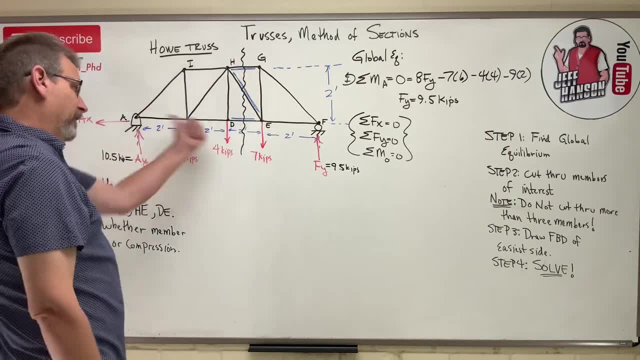 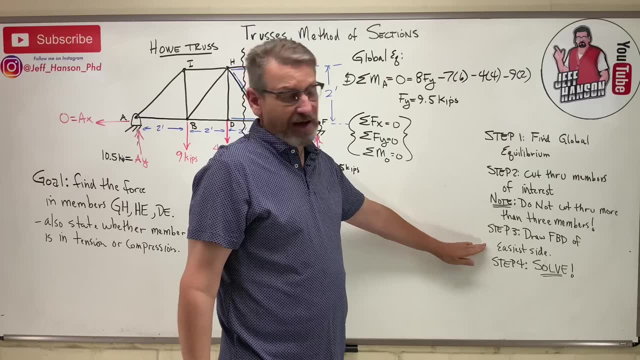 two, three, all right. So draw the left side or the right side. Next one says: draw the free body diagram of the easiest side. I tell my students be lazy, okay, Draw the easiest side, And it doesn't matter which one you draw, you're going to get the exact same thing. So 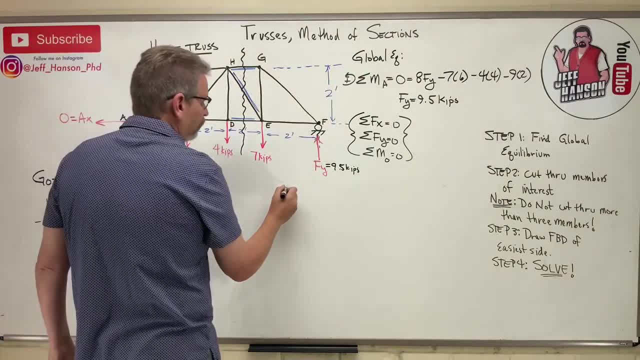 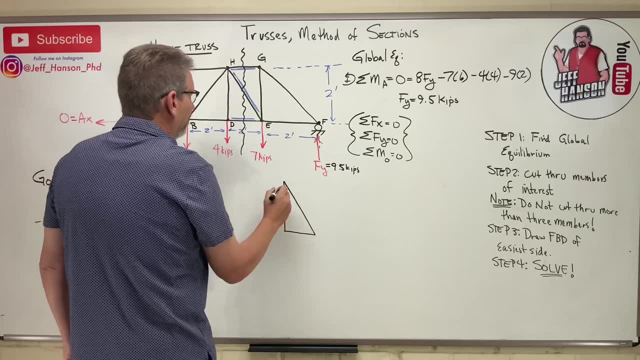 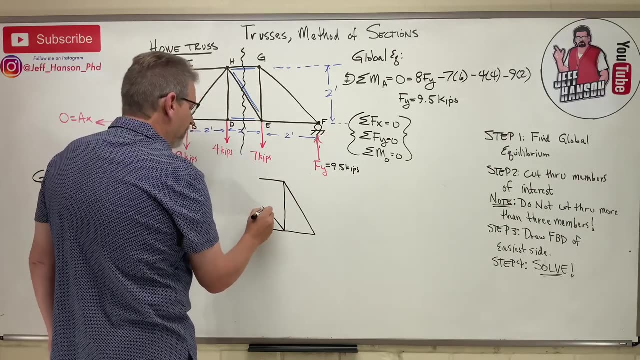 let's draw that side over there, okay. So I'm going to draw that free body. Here's this triangle and then it has a force here, one here and one there. So there's my three members Now. on the method of sections, I don't generally try and get these directions. 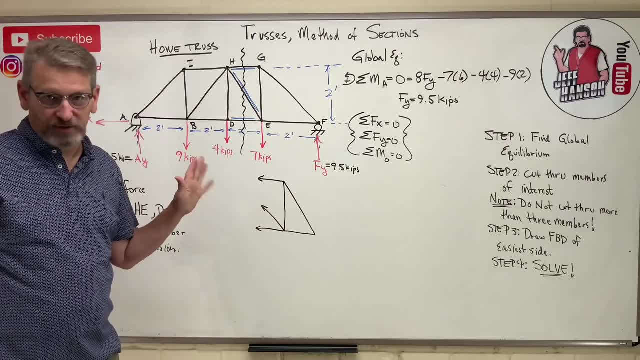 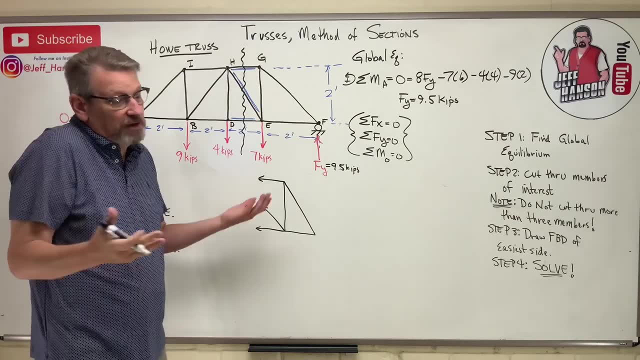 correct. I always guess them all in tension and then we'll let our math sort it out. If I get a negative for one, then hey, it was really in compression. I guessed it in tension, it was really in compression, No big deal. Now let me put the other one in. I'm going to put the other. 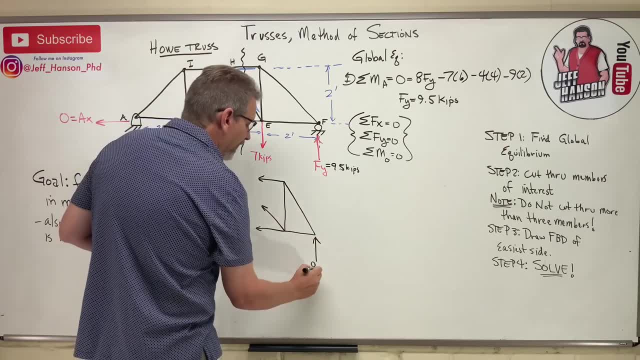 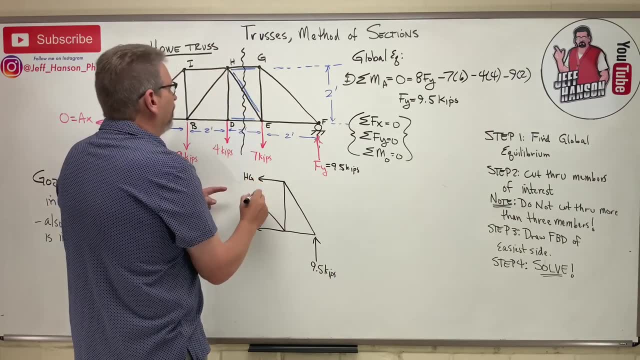 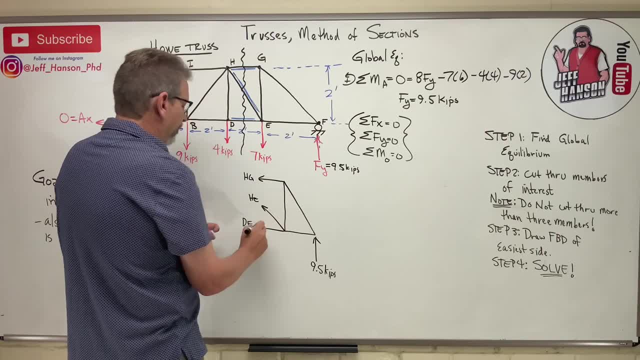 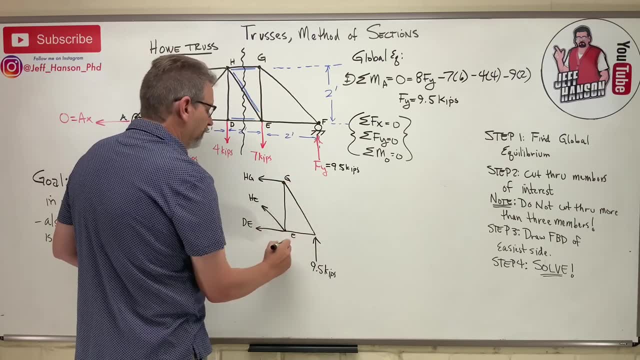 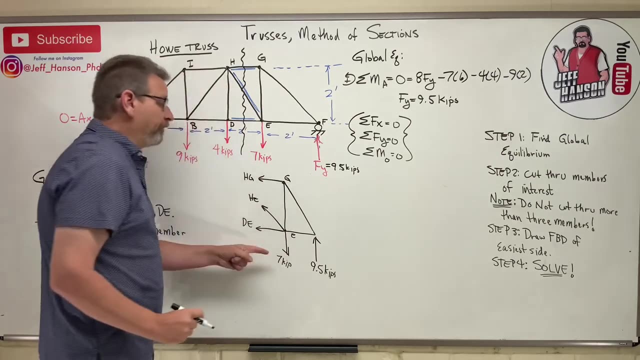 and this guy is DE. Okay, So let me do, I'll just label these: This is G and this is E, okay, And then also there's a 7 kip right there. So any force on here, I'm going to put it in compression. So I'm going to put the other. 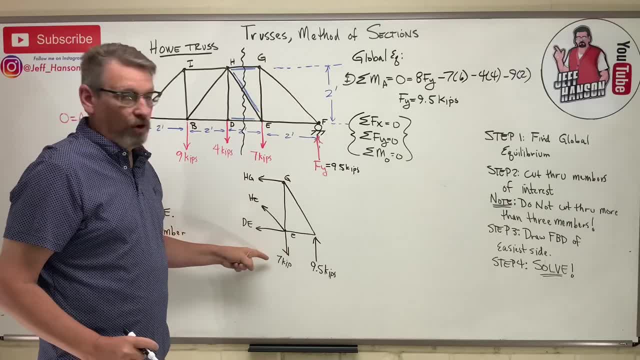 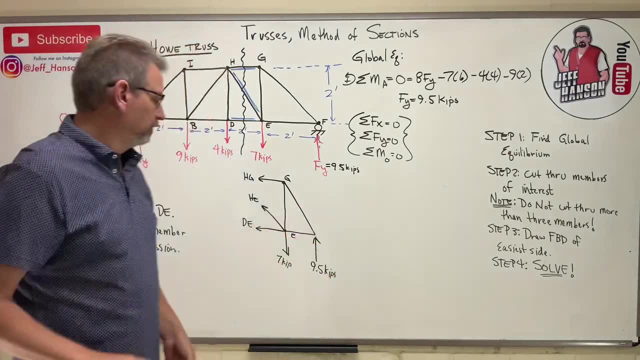 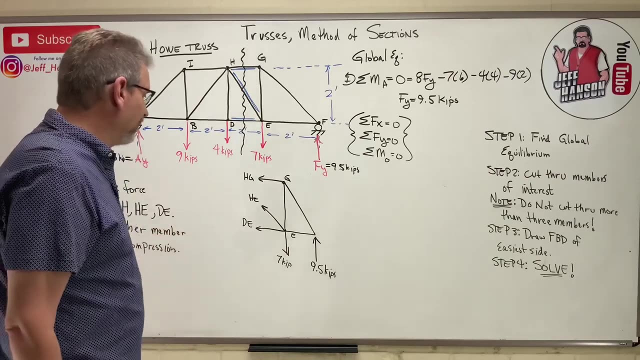 forces on that side of the truss that I draw I have to put on my free body all of them. Okay. Now the next step says solve. Well, yeah, because look what you've got here. This is just a little old, normal statics problem, just a regular old statics problem, okay. So 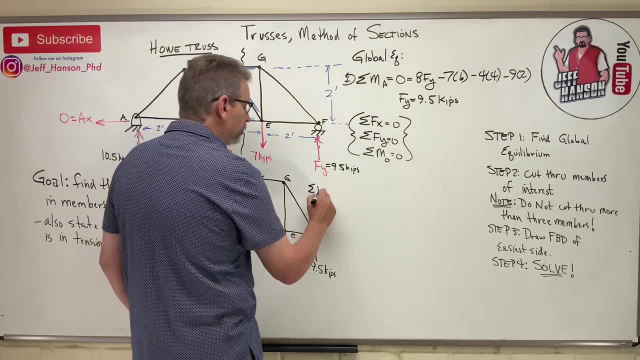 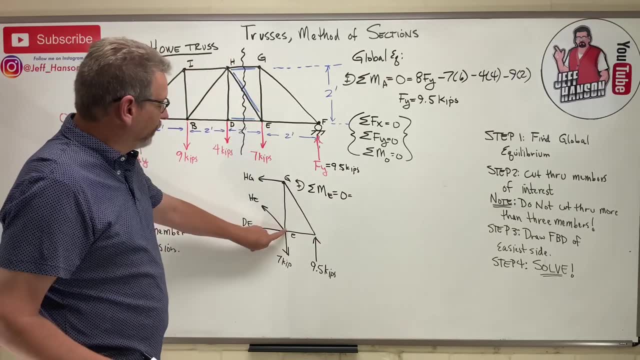 if I take the moment at point E, this being positive, what do I have? Who gets knocked out? if I take the moment at E, I'm going to put the other forces on here, So I'm going to put the moment at E. Well, the 7 kips gets knocked out, DE gets knocked out, HE gets knocked out. 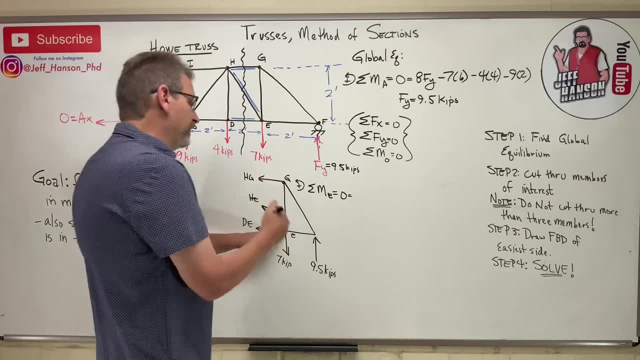 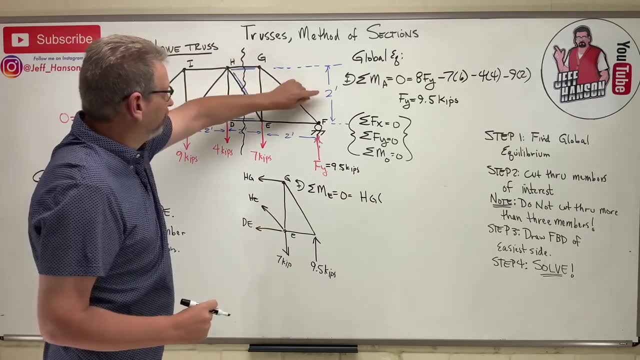 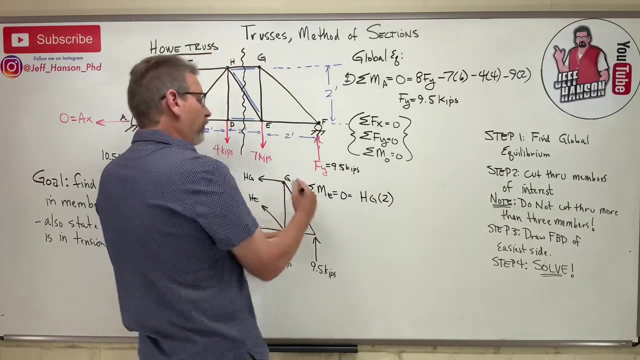 and the only one left is HG, which rotates me positive. So HG times, how far away? Well, from point E all the way up to there is 2.. And then I've got this guy, this 9.5,, which also rotates me positive. And how far away is that guy? Well? 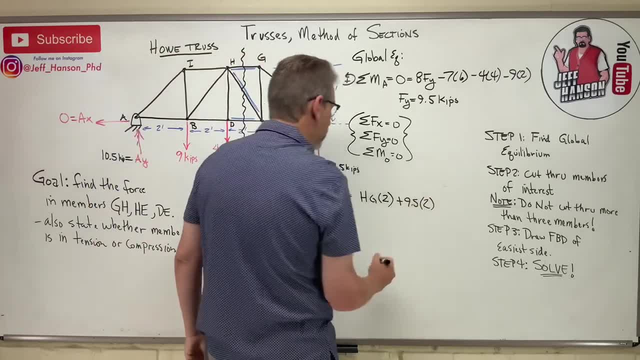 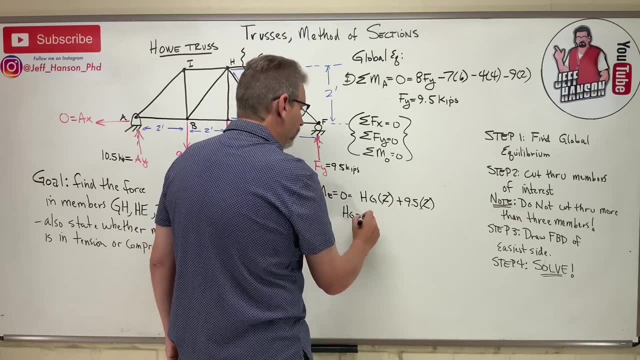 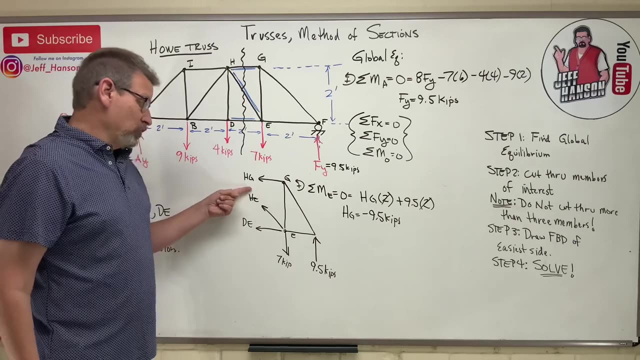 he's also 2,. okay, So I can divide everything through by 2, and I get: HG is equal to negative 9.5 kips. okay. So what does that mean? That means that I assumed HG in tension. 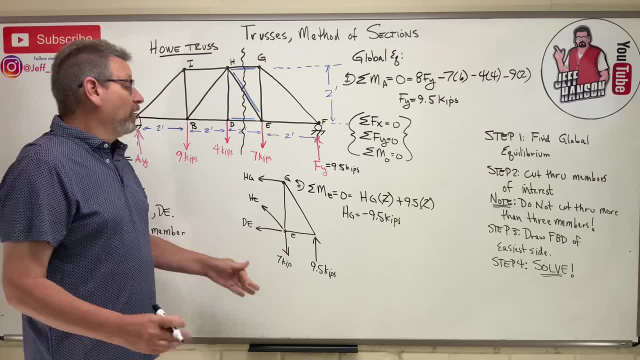 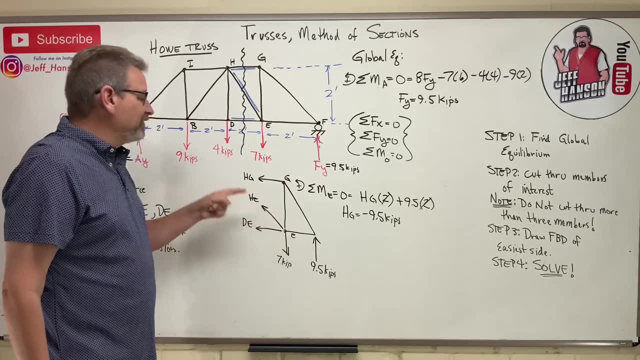 but HG is really in compression Now. you can leave it alone, You can leave it just like this. and then every other equation that you write from here on out every time you use HG you have to put in negative. For me, I think that leads my students to a lot of mistakes. So 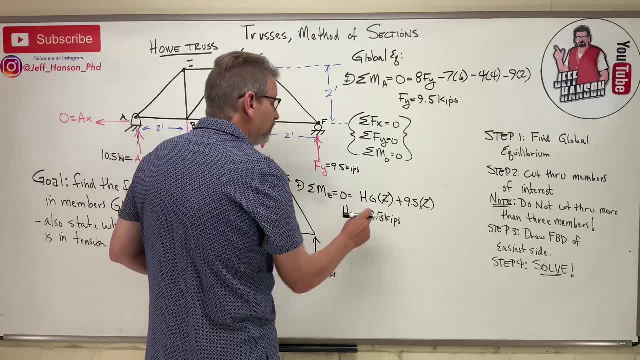 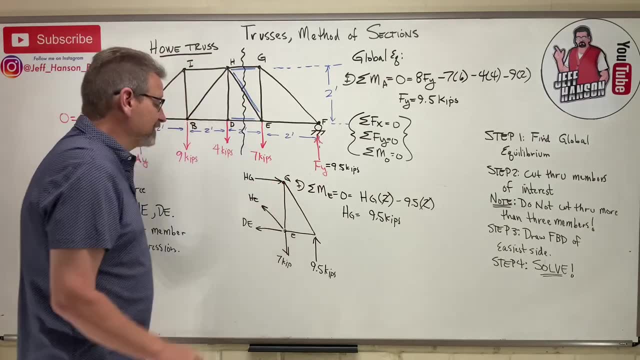 what I would say is, when you get a negative right, go ahead and fix it. okay, I'm just going to, I'm going to fix it right. A lot of people would say: just leave it alone and put a negative in. 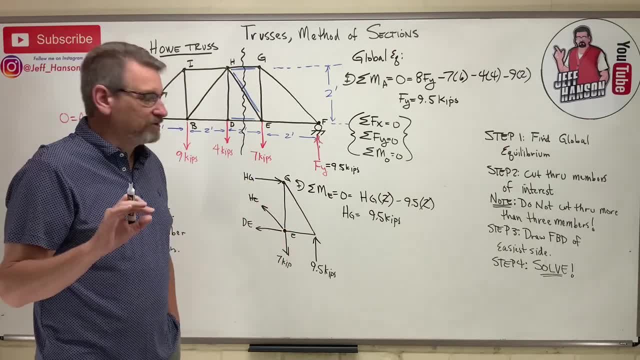 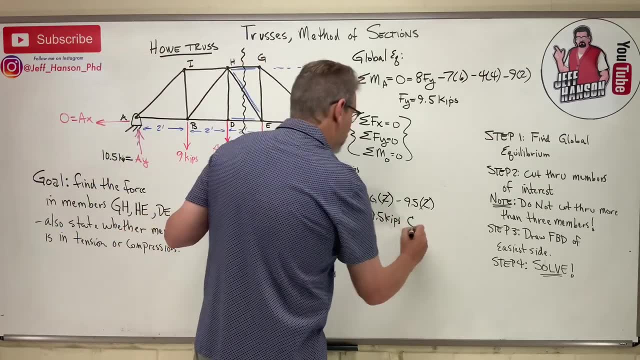 I think it's better you'll have less errors if you just fix your free body diagram when you see one that's backwards. So there's HG, He's in compression And you'll notice. well, I should have done this. I should have left him a positive and made him a negative. 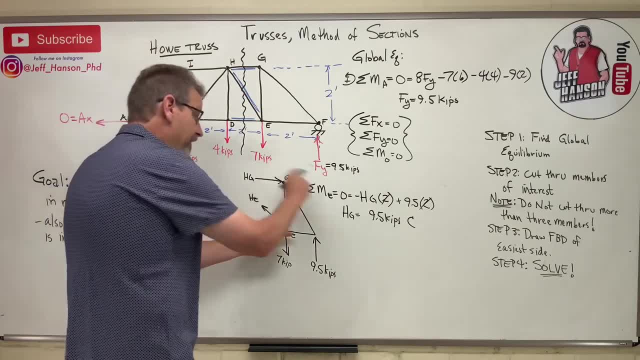 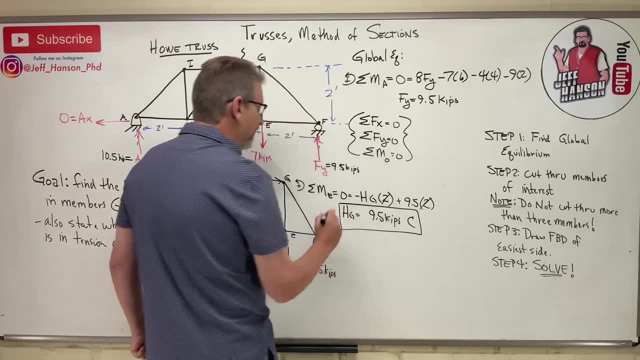 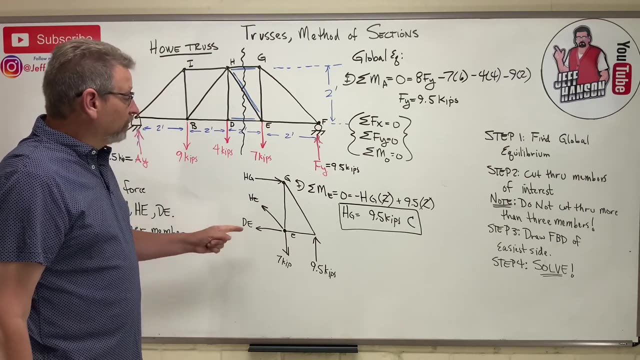 right. So because he's going the negative direction, which is causing a negative rotation, and now it's fixed. So there's HG. That's one of the three things that they asked me to find. Okay, that was good. Now what? Well, now I can do. I can just do something simple here. 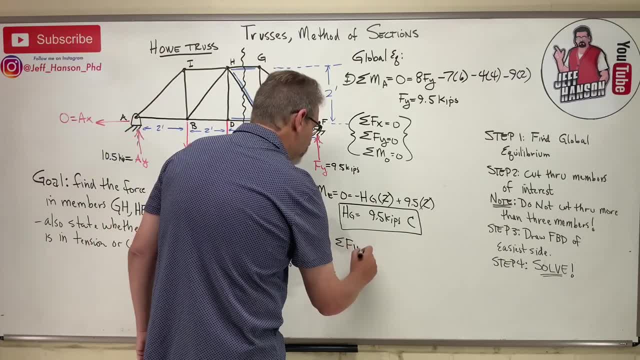 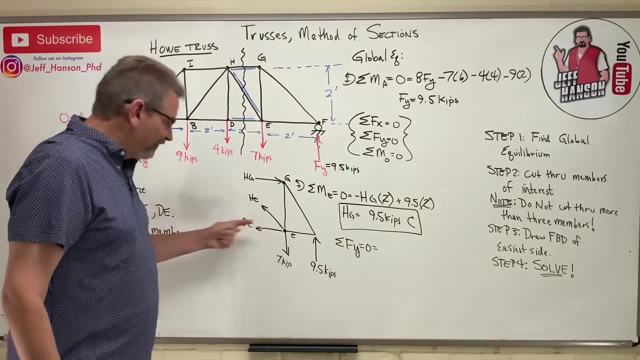 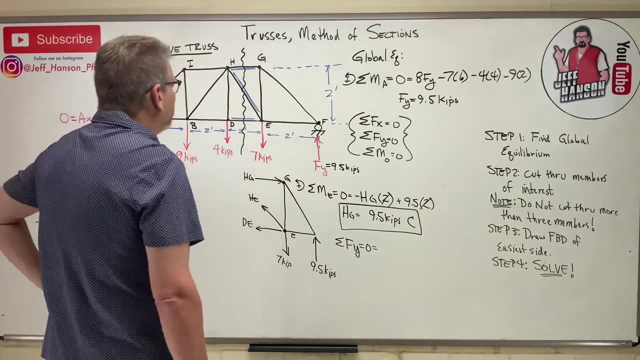 and I can do this- The sum of the forces in the y direction. okay, I like the next equation to note in it. And since DE is in the x direction, he's not going to be in the y equation, So the only one in the y equation is going to be HE. Oh, you know what we need there? We need an angle. 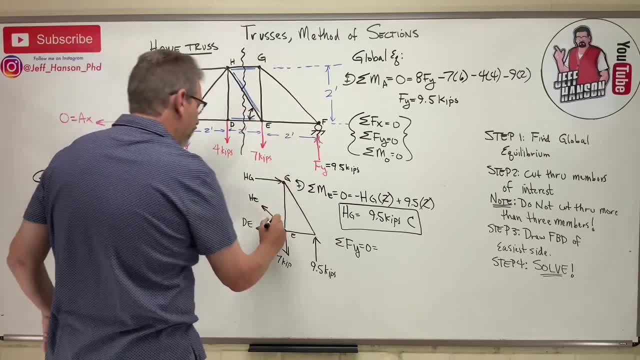 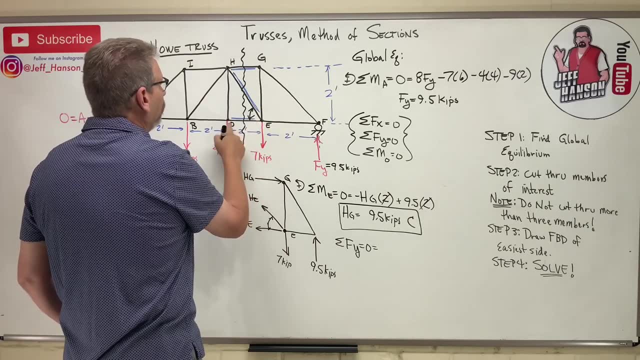 don't we? We need this angle right here. okay, This angle right there, And we've got this little triangle. that's one on this side. No, sorry, It's two on this side. Oh, it's two on that side. 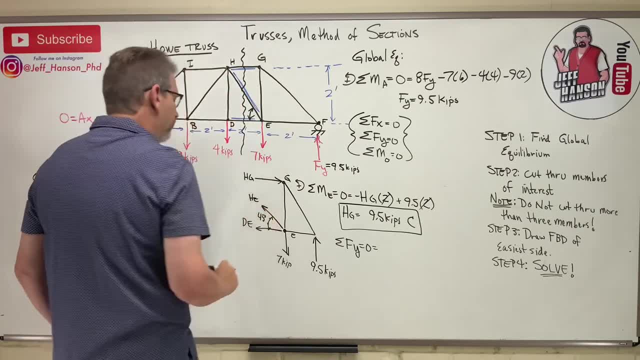 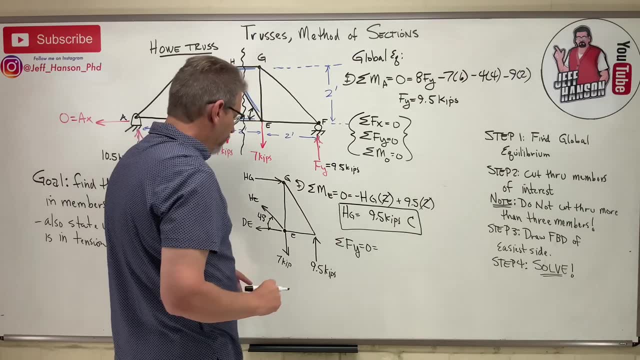 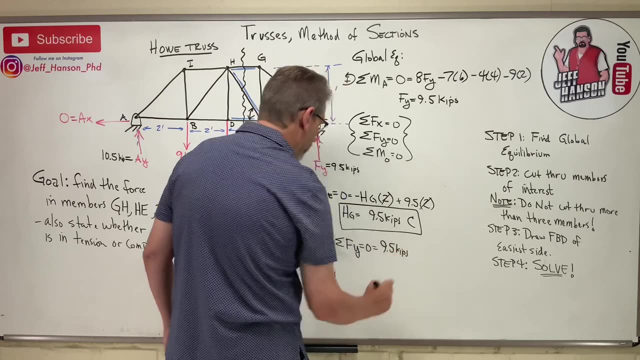 I know what that angle is, don't I? It's 45 degrees, isn't it Okay? So, in the y direction, what do I have here? Well, I've got 9.5 going uphill. Okay, I've got seven kips going downhill. 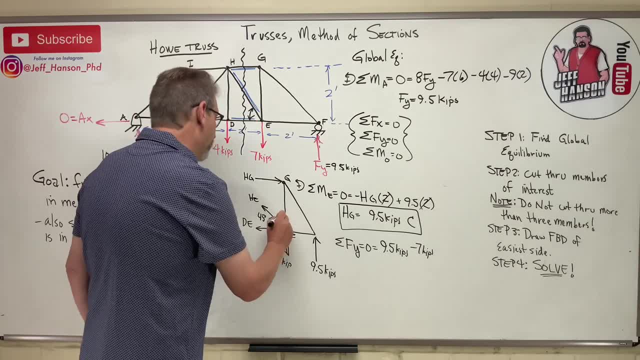 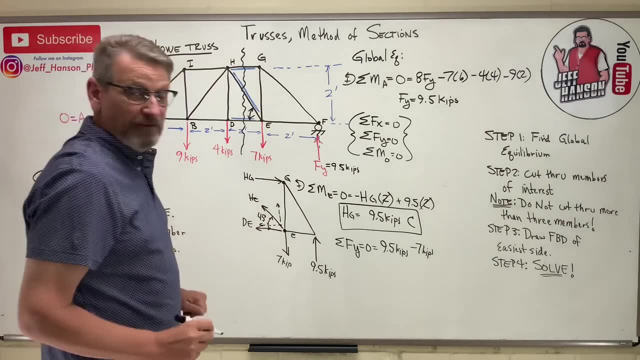 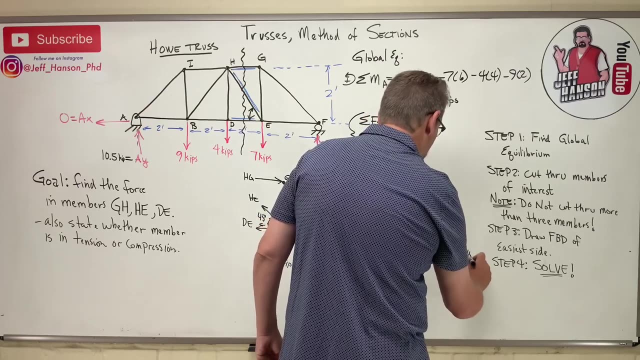 And then I've got going uphill over here. right? This guy has two components, and the y component is HE sine 45, and that's going uphill. So plus HE sine 45. Looks like my direction is going to be backwards again, doesn't it? 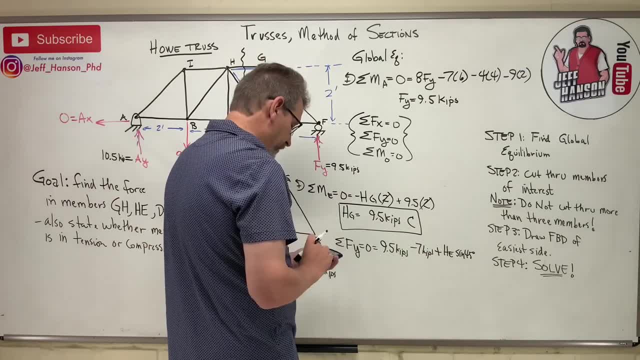 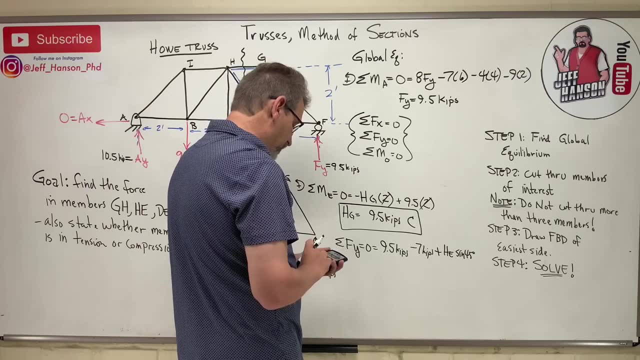 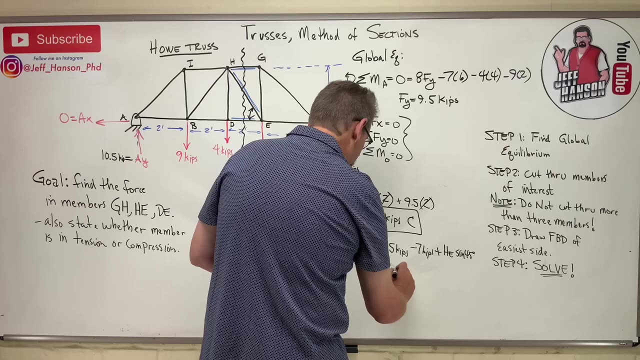 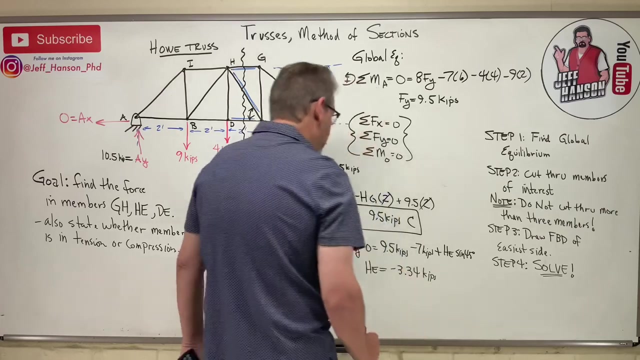 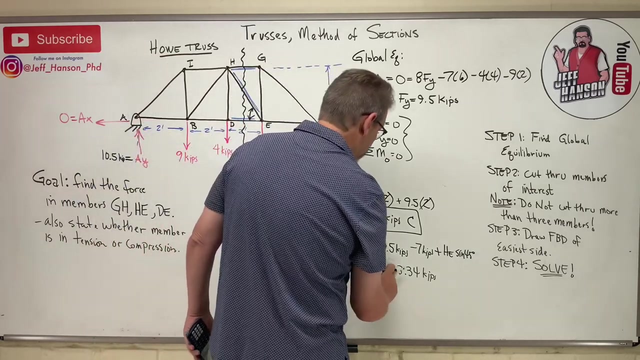 Okay, So move the seven to the other side on. seven minus 9.5 is negative 2.5 divided by 0.707.. So HE is equal to negative 3.35.. Okay, I guessed him in tension. Guess what He's really in compression. okay, Really and truly. 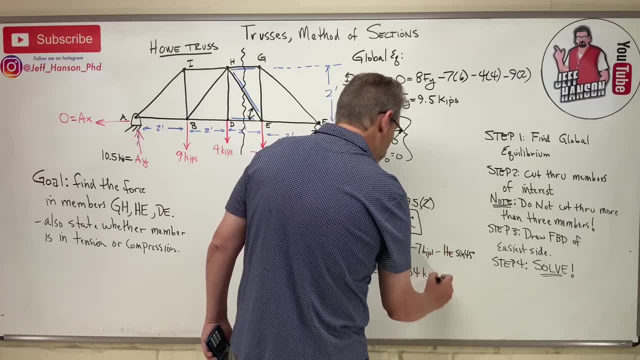 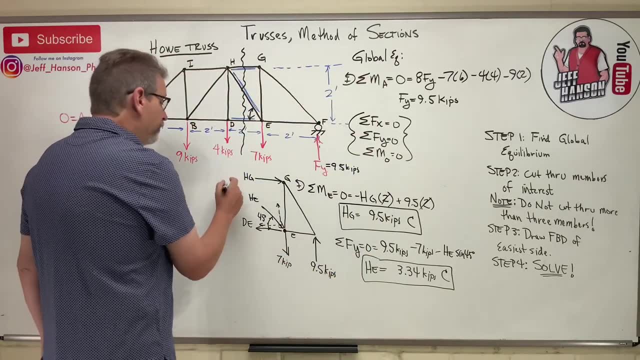 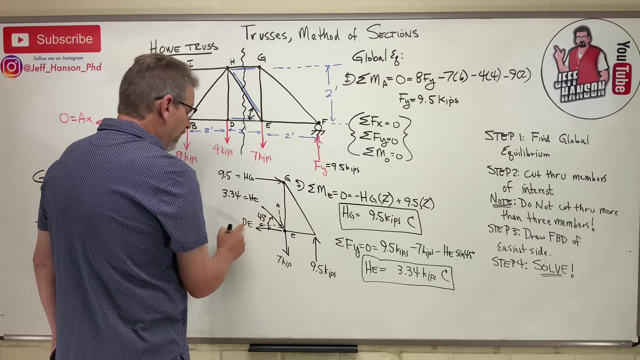 he's in compression. I'm just going to change that to a negative Compression, All right, So now, I know you, This guy is 9.5.. I know you, This guy is 3.34.. And I'm looking for you. 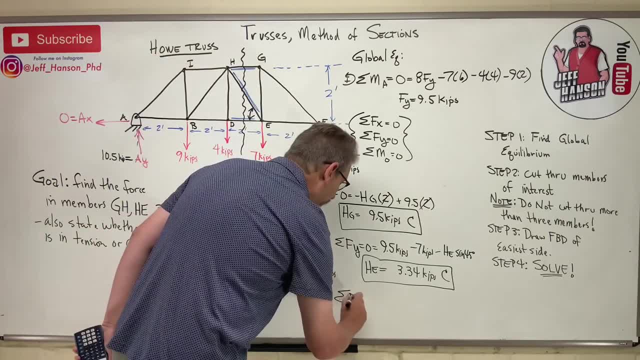 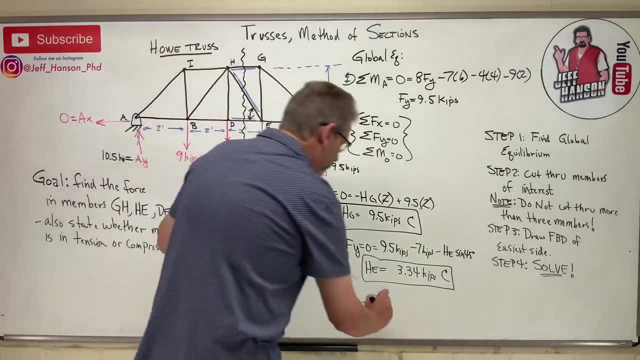 All right. So I've got negative 2DE, That's easy. One more step: Some of the forces in the x. And what do I have in the x direction? I have HG which is 9.5.. And again, if I didn't correct that, I would have had to leave it in the negative direction. 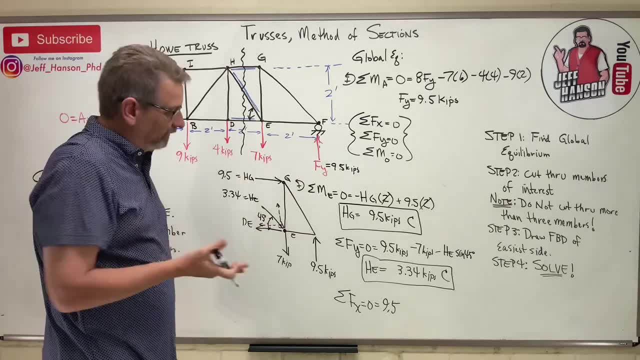 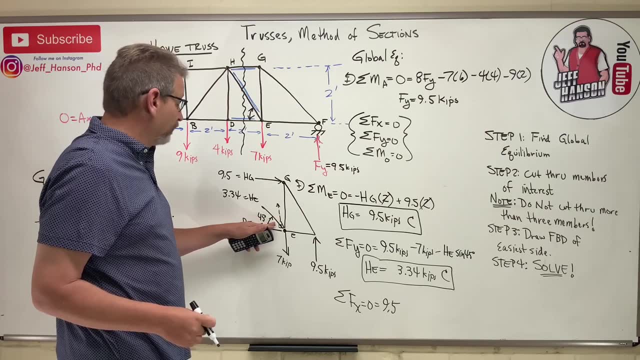 So I would have had to have a minus, a minus And see that's just confusing. It's easier if you fix it, I think. All right, In the positive x direction, I have this guy: 3.34.. 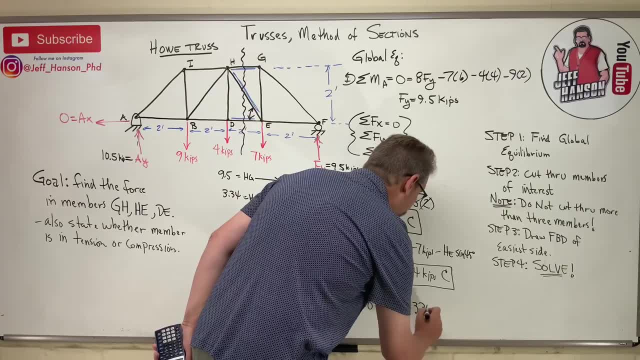 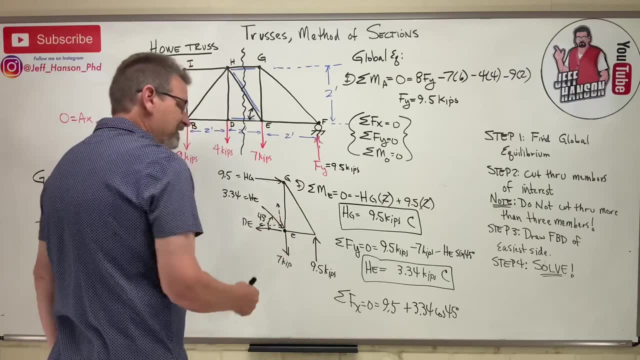 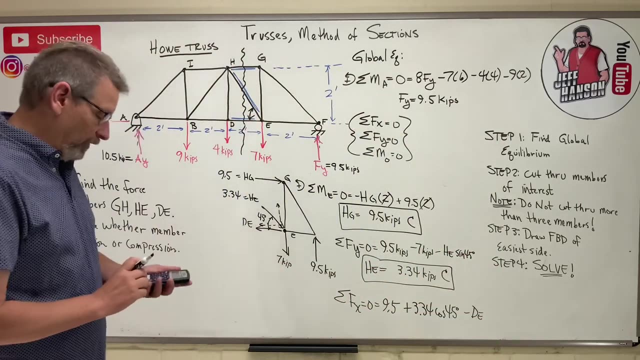 So plus 3.34 times the cosine of 45. And one more is DE, And he's in the negative direction. Okay, So I guessed all three of them. It looks like DE is the only one I guessed, right. 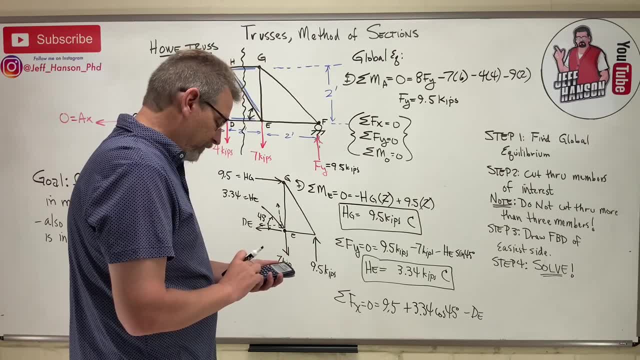 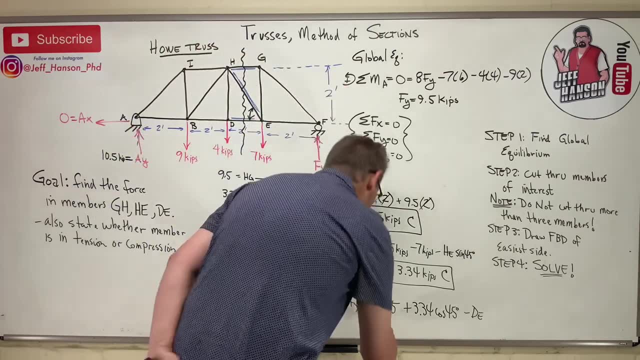 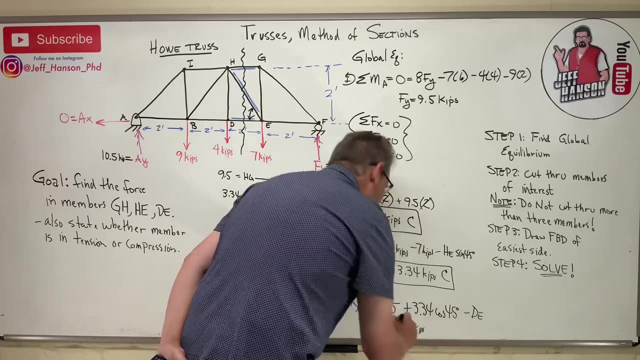 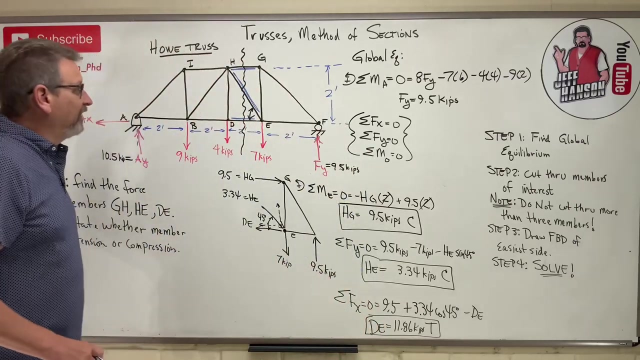 So 9.5 plus 3.34 times 0.707 is 11.86.. So DE 11.86 kips. And guess what? That one's in tension. Okay, And that's it. That's the method of sections. 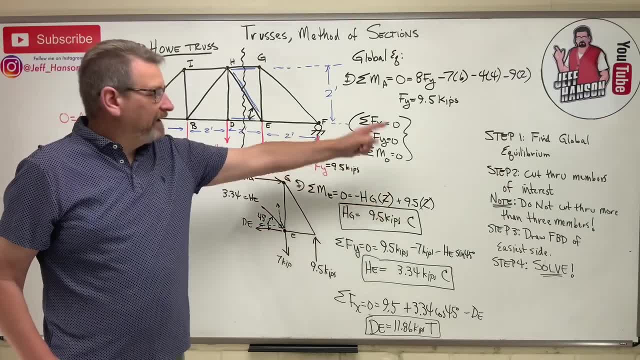 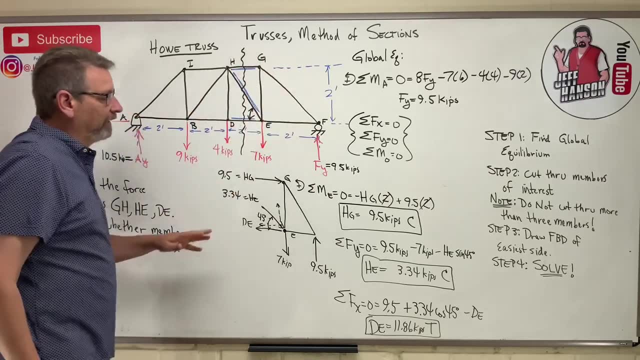 So if you follow this simple little recipe I have for you over there, man, these problems are easy. Just cut through the members of interest, take it apart, draw the free-by diagram to the side. Now remember this. You don't find anything. 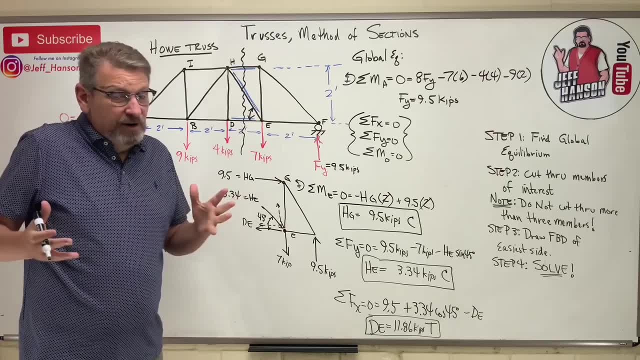 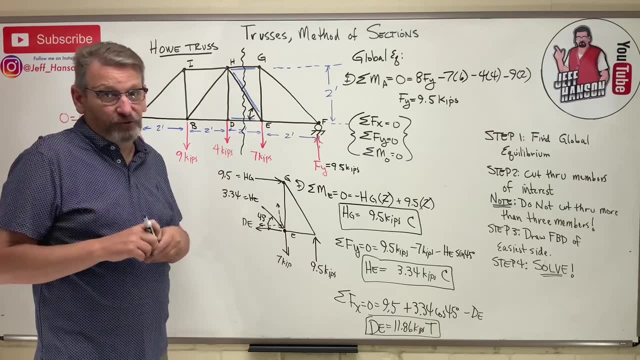 You're not going to find anything out about these ones that you didn't cut. If you don't cut a member, you don't find out what's inside of it. So don't worry about the ones that you did not cut, because the sum of the force in those is zero and you're not going to find anything out about them.